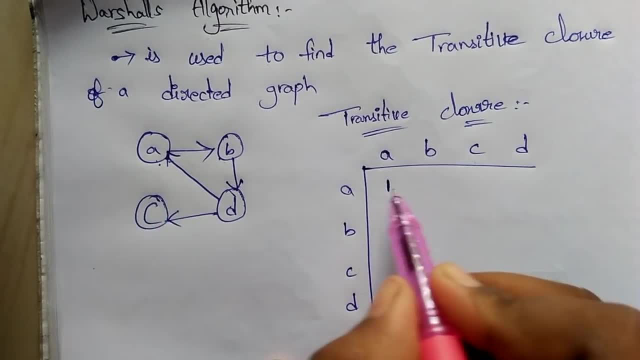 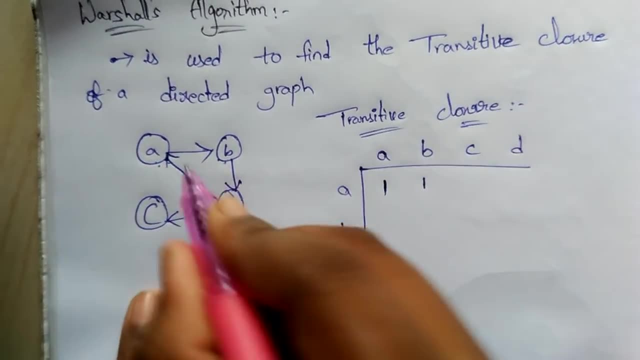 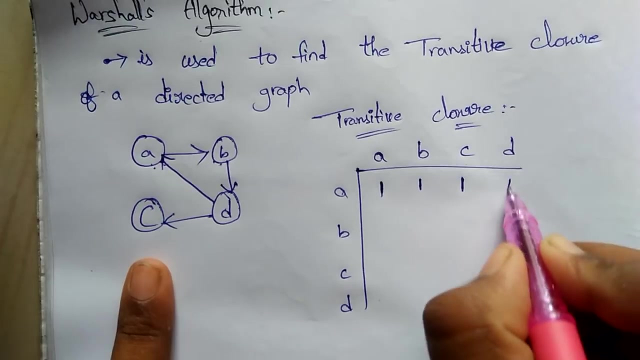 D, D to a. there's a path from a to A, okay, so then there is one next B to A to B. sorry, there is path, so one A to C, A to B, B to D, d to c. there is a path next a to d, a to b, b to d. okay, there is a path next same. uh, how same we need. 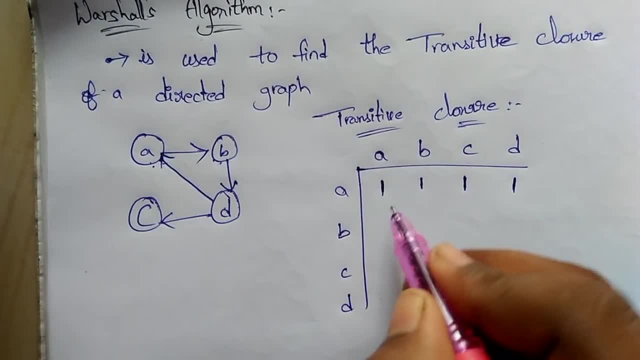 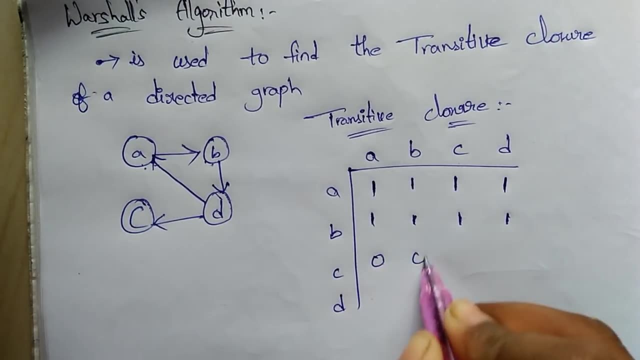 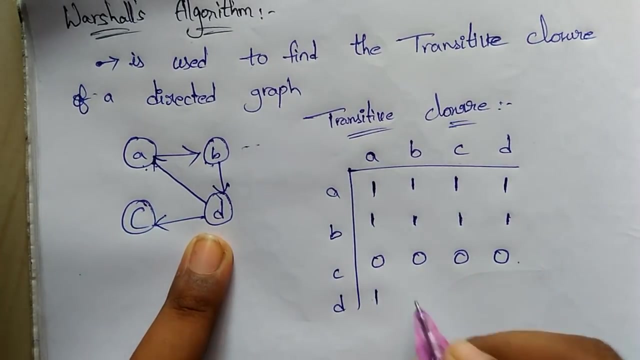 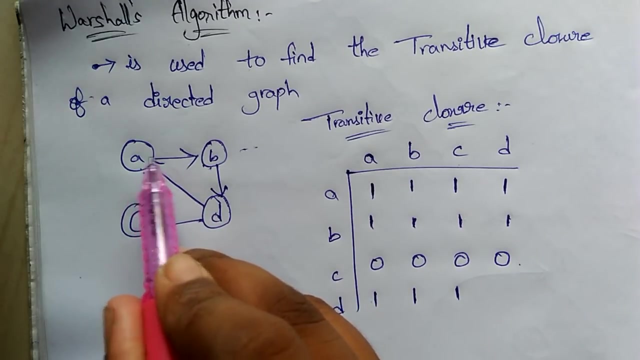 to write for b2. okay, so b means one, one, one one. so you need to draw this. so c have no outgoing edges, so it's all zeros and d again. so there is a path from d to a, next d to b, d to c and d to d. how means? a to d to a, a to b, b to d again. so okay, this is a transitive closer, we just 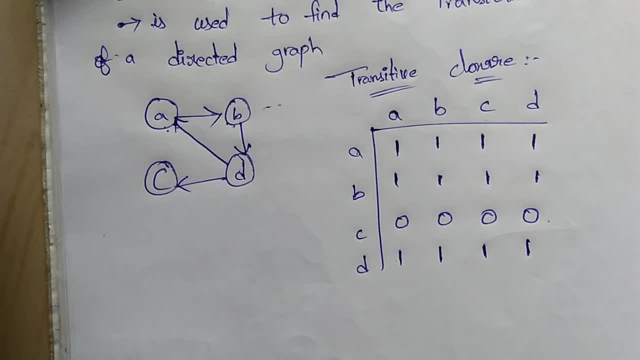 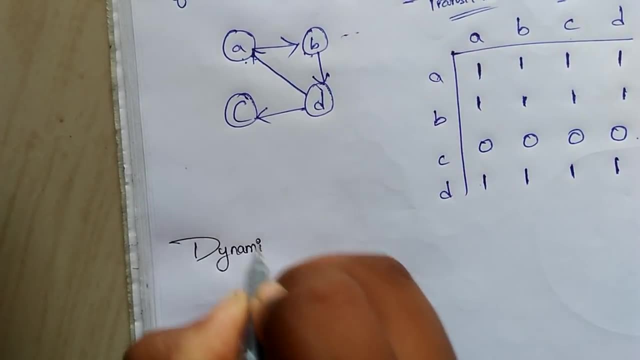 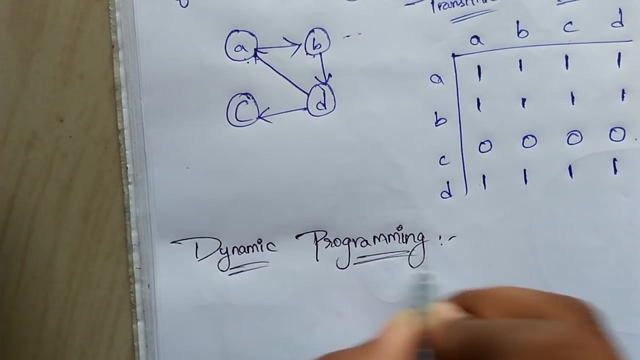 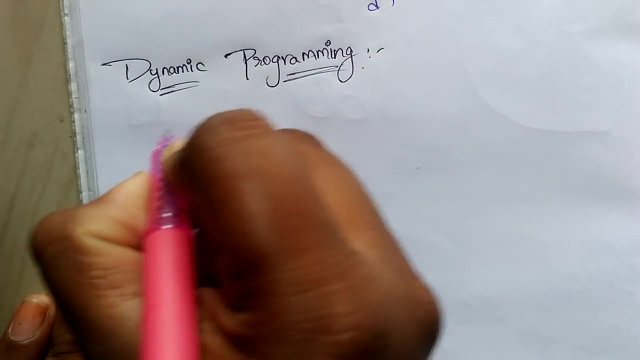 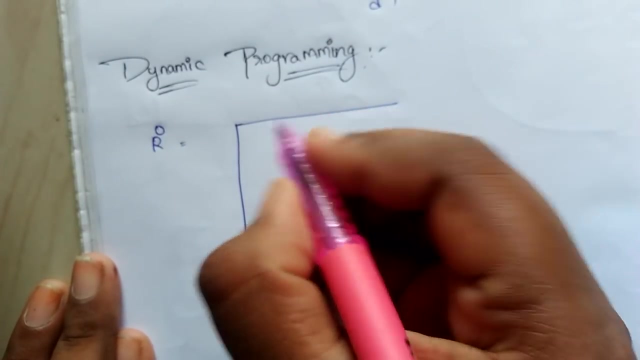 wrote very simply, but we need to find this transitive closer using dynamic programming next. next we need to. we need to apply this all over them to the given directed graph using dynamic programming. okay, so dynamic programming means we need to. first we need to calculate r power zero. r power zero means, so take the adjacency. 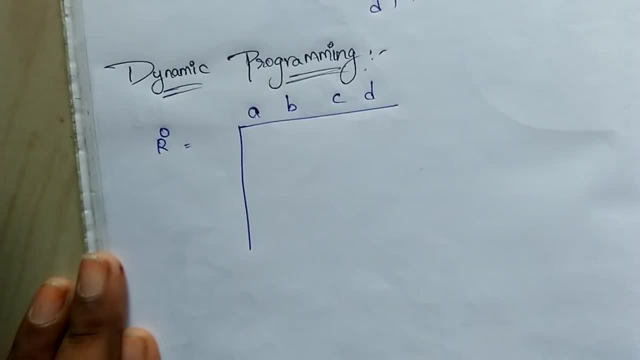 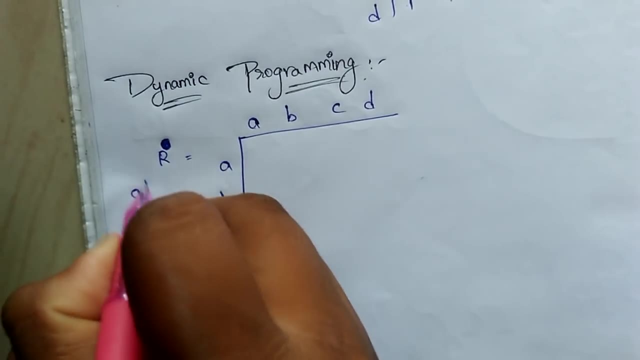 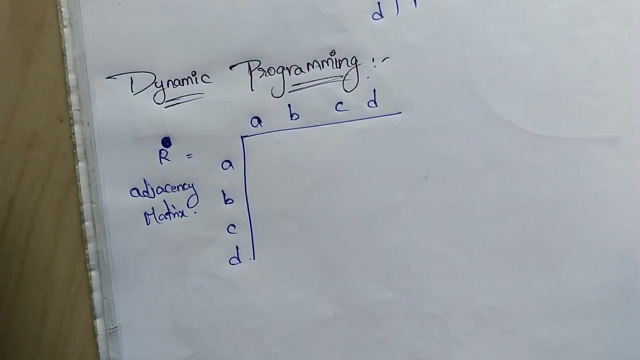 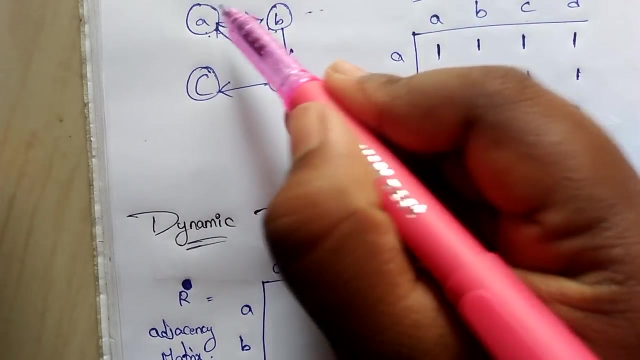 matrix. okay, so adjacency matrix. first r- i'm calculating r- means adjacency matrix. so adjacency matrix means there is a direct path. so how we'll write the directed path means: okay, i think you can see both. so there is. is there a direct path to a? to a? no, so there is zero. 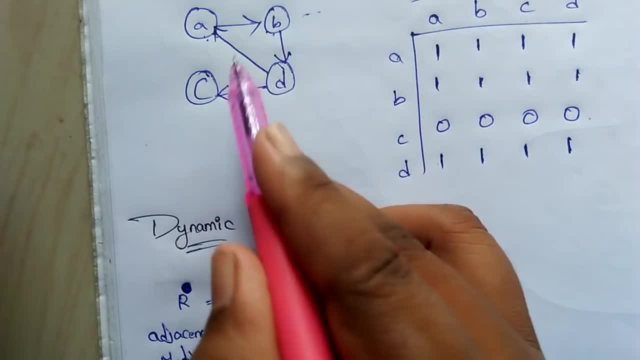 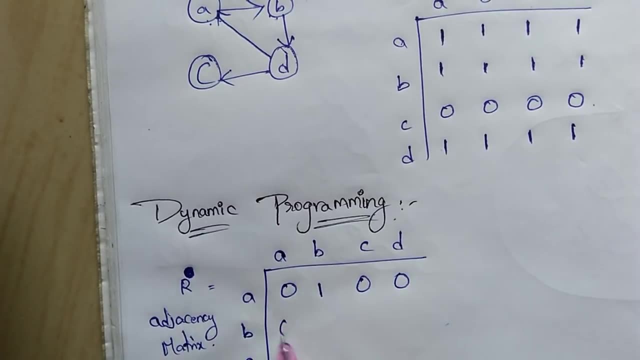 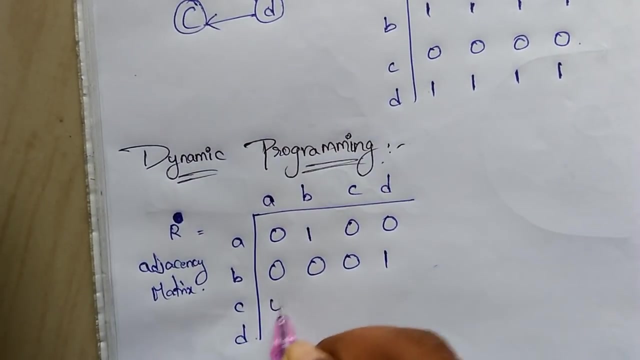 there is a direct path from a to b, so one a to c. there is no direct path, so zero. next: a to d, no b to a, no b to b, no b to c, no b to d. there. okay, so in this way we write the adjacency. 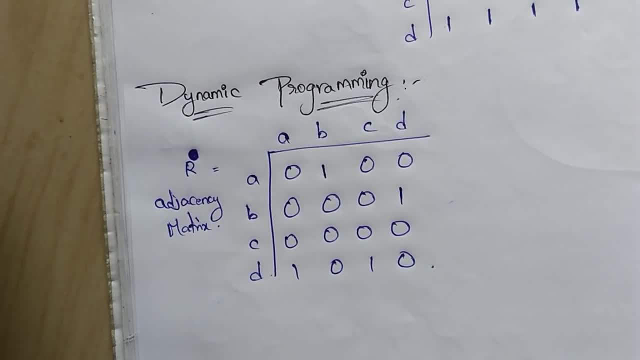 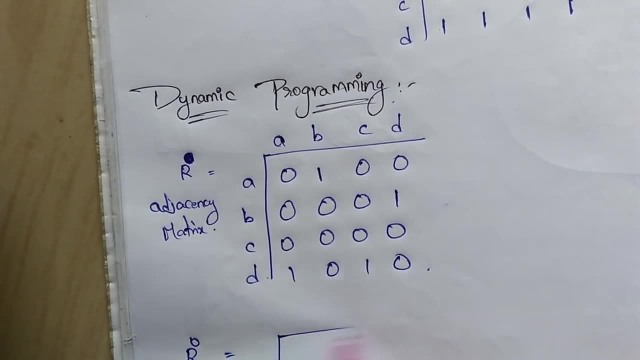 matrix. okay, let's apply this washer's algorithm to the given adjacent matrix. next, first, r of zero. okay, so r power 0 means we just mark all the first row elements and the first column elements. so what means a? i'm just writing the above matrix here, okay. 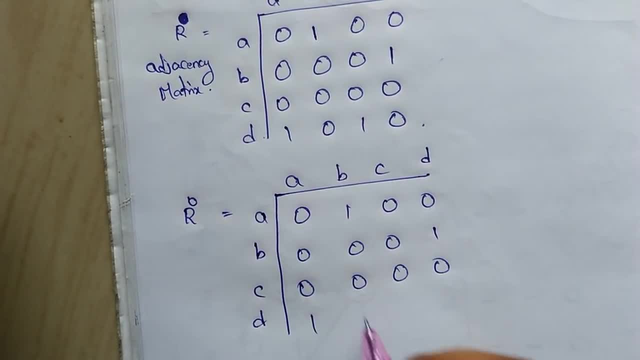 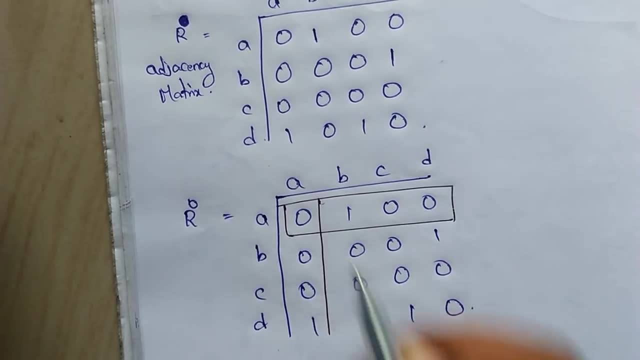 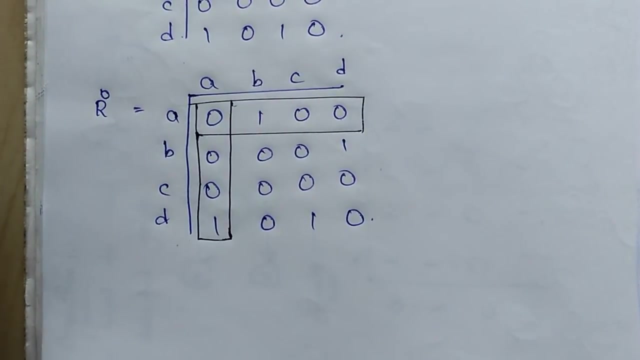 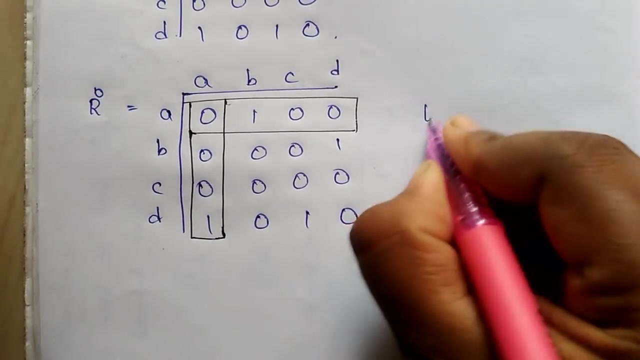 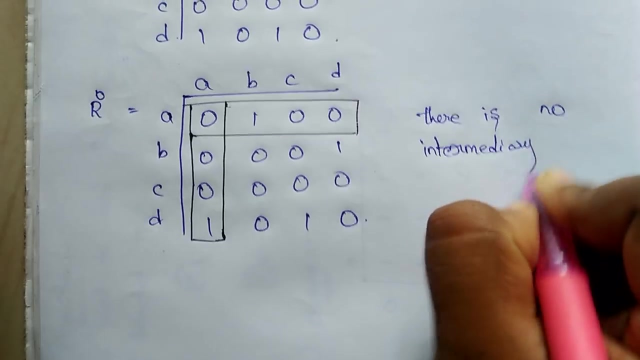 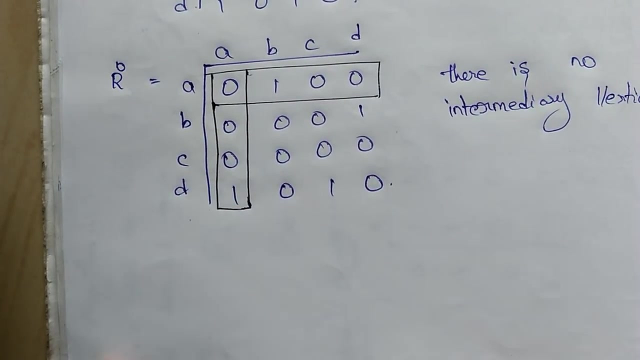 00010014 zeros, one zero. so we need to mark. okay, we need to mark this and this row and this column. okay, here there is no intermediary vertices. here, there is no intermediary vertices. okay, next, by applying, how will apply? so let's here. it is a crucial in this water zone. over them, so please. 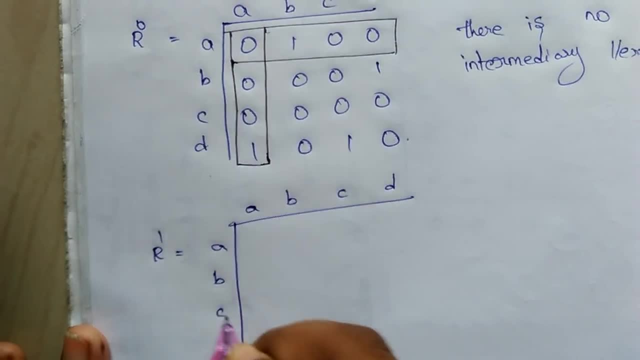 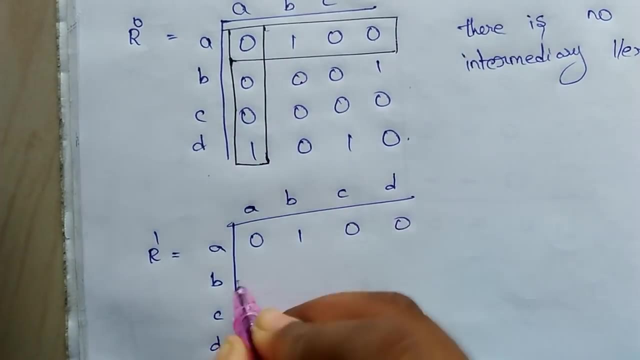 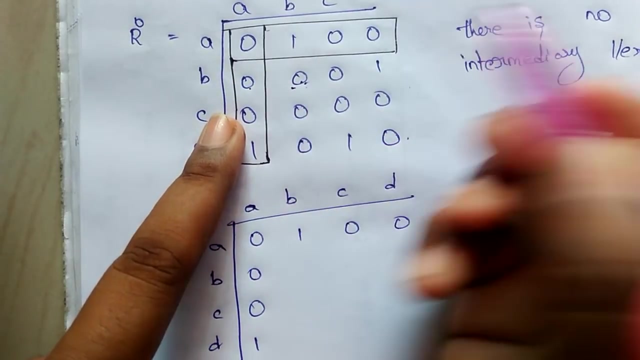 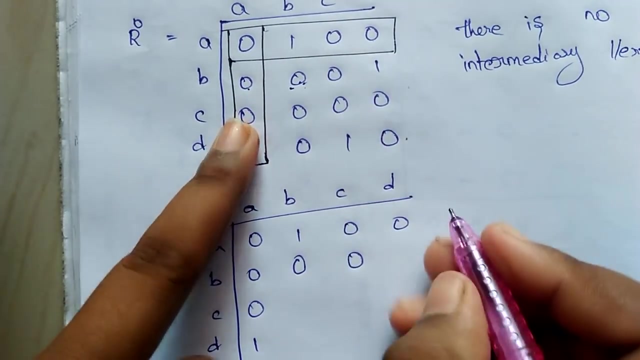 be concerned related here and here we need to be. don't change this. I'm writing it normally. what we need to do is we need to change these elements and that's it. so here is zero and here is one different element, so we need to place zero there. okay, you're 0, 0, 0, 0 and 0, but here is one we don't. 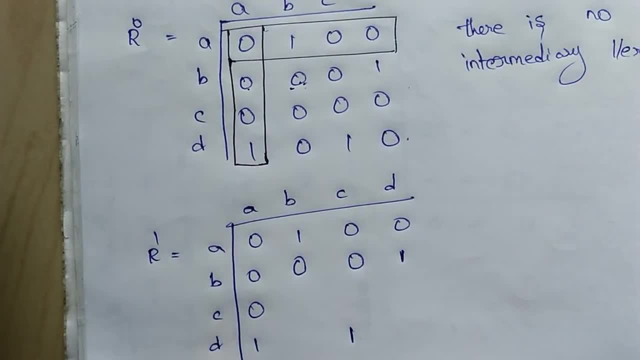 need to change one here. here also one. we don't need to change those. so 0 and 1,. here also 0, 0 and 0, 0, 0 and 0, 0, 1 and 1, here we are changing 1, please. 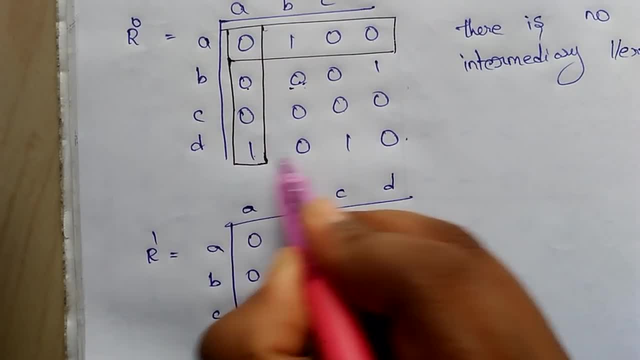 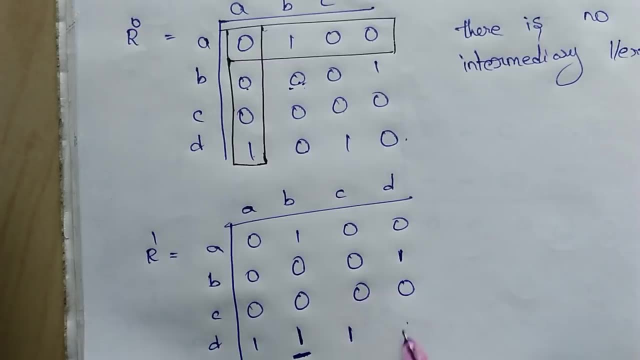 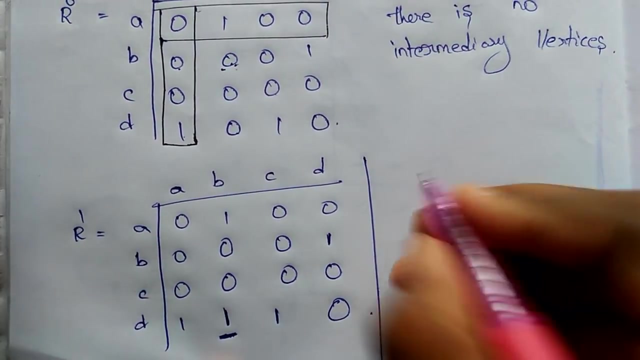 be concentrated here, okay, because here the selected row and selected column gives 1 value. so we are placing 1 here, and here is so 1 and 0, so here placing 0, this is R1 step. so here we'll write R2, same. okay, I'm just writing, please write it down- so R2, R power. 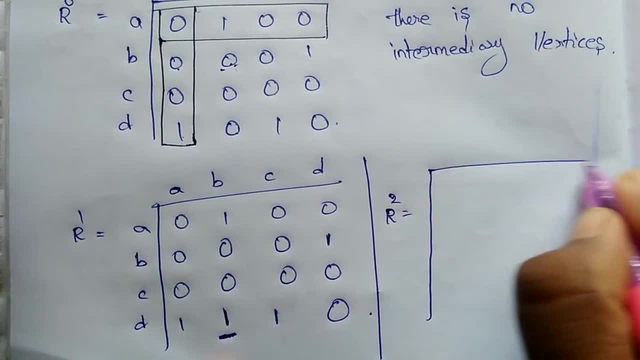 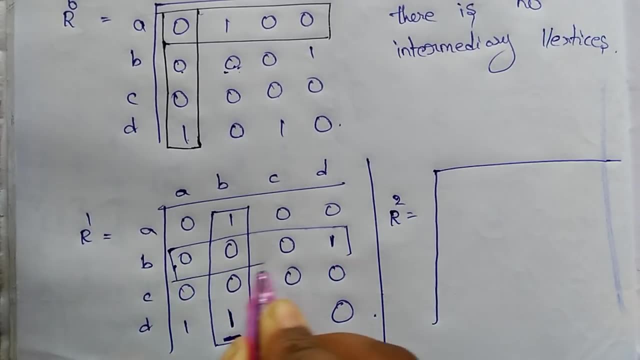 2,. okay, not R square. okay, so the same notes here also. next we'll mark the second row and the second column. that's it. okay. here is 0 and 1, so we need, we no need to change.